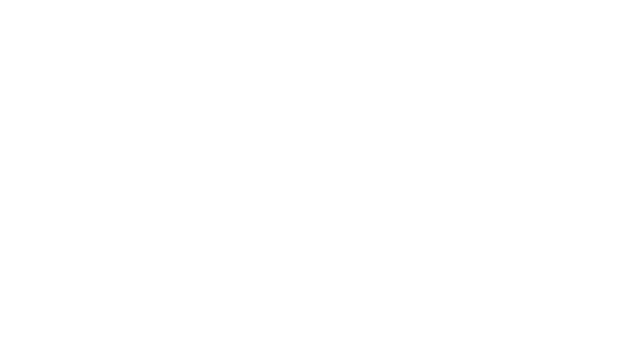 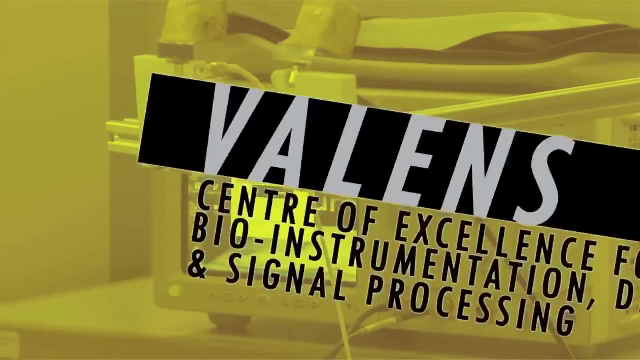 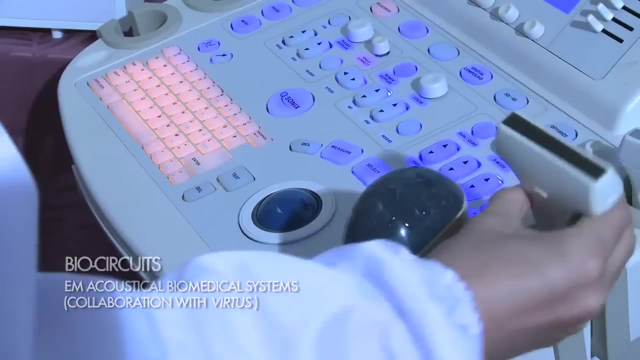 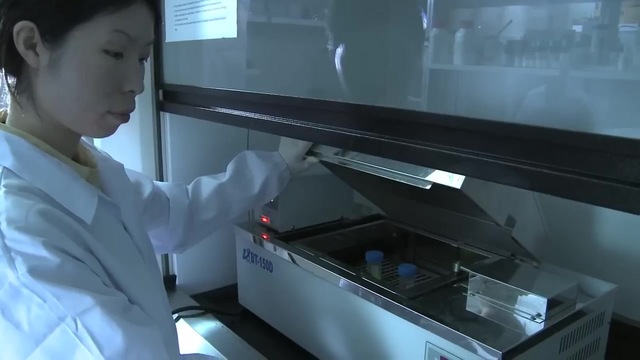 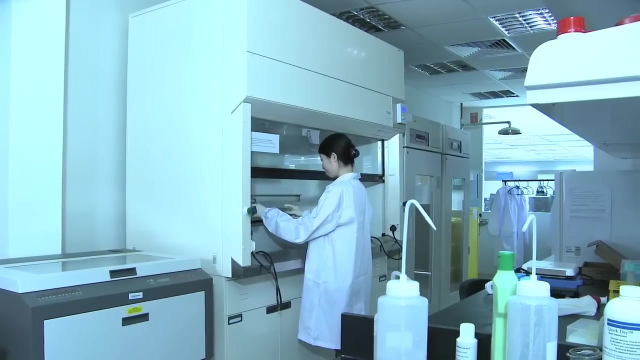 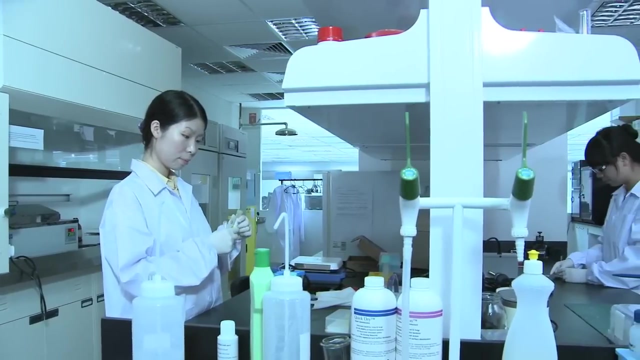 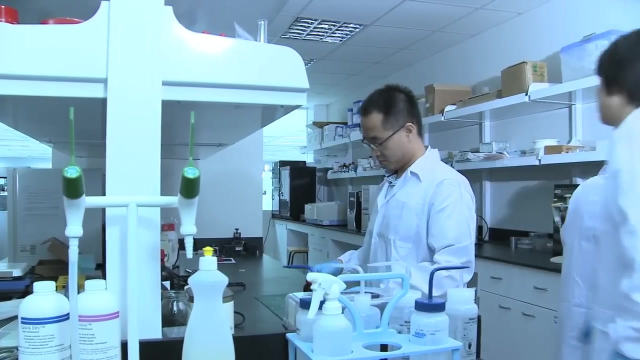 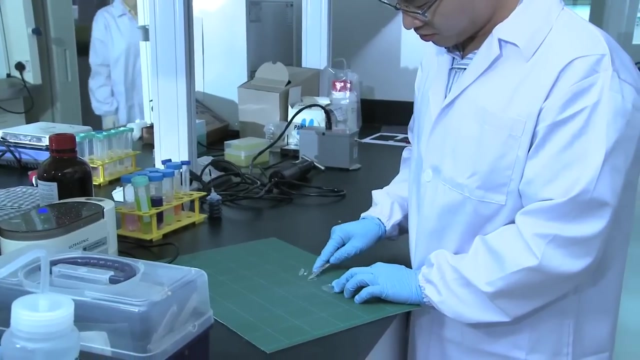 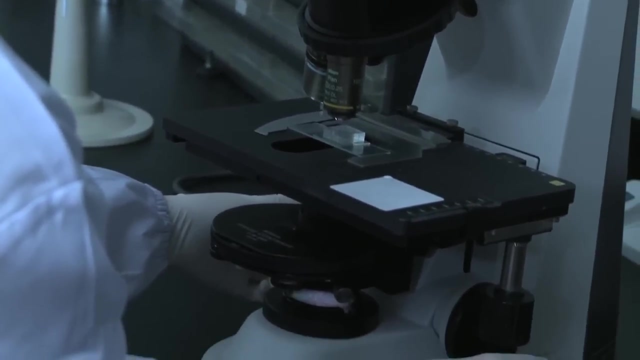 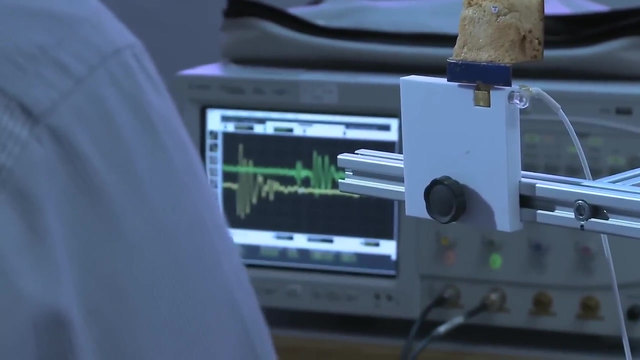 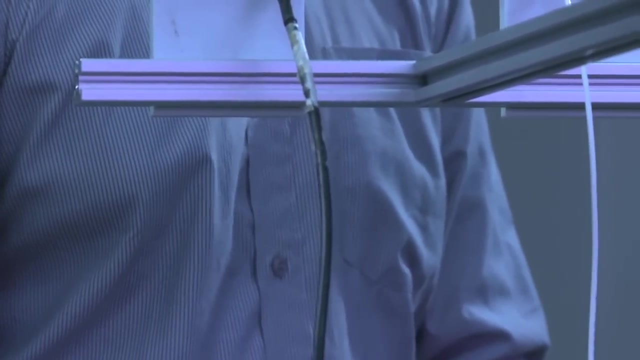 Transcription by CastingWords. Transcription by CastingWords. Many of our research projects are inspired by clinical needs. One of them includes the Ultra Wideband Respiratory Monitoring System. Transceivers are used to observe chest wall movement for the detection of abnormal breathing patterns and sleep apnea symptoms. 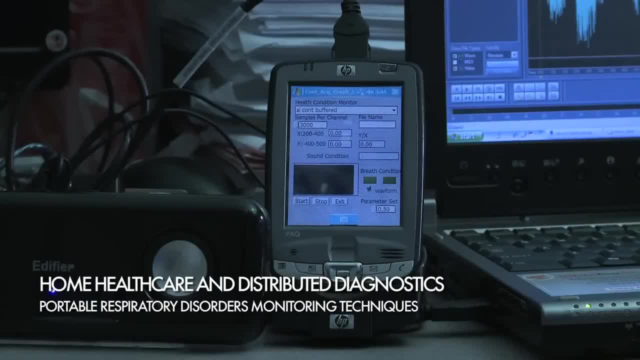 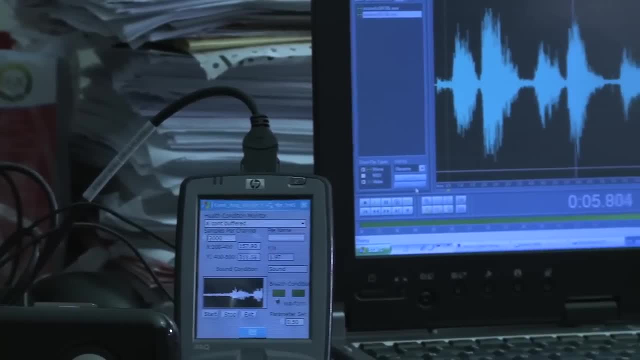 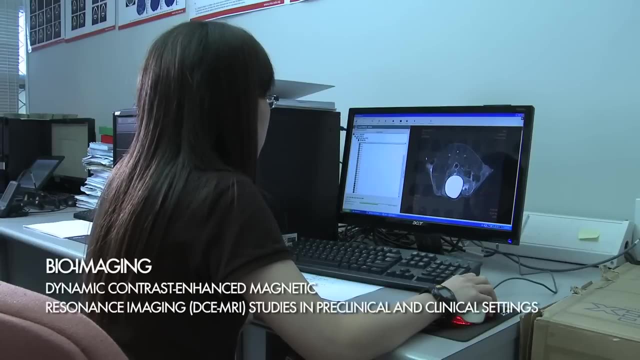 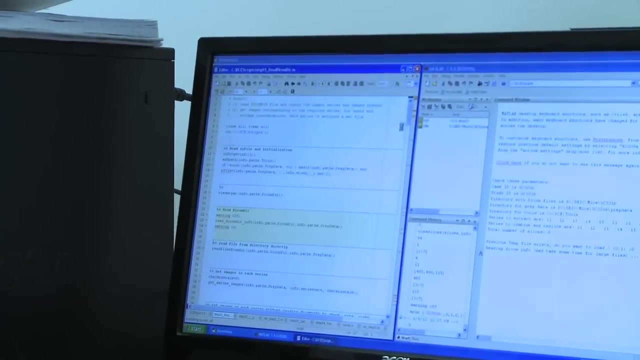 Our joint venture with National University Hospital has developed a portable respiratory disorders monitoring technique. This compact device uses sound-based technologies for respiratory disorders monitoring. In another collaborated venture with the Singapore National Cancer Centre, the Bioimaging Project has developed a tracer kinetic model. 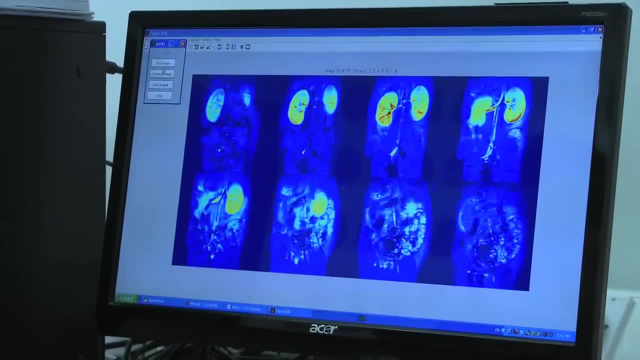 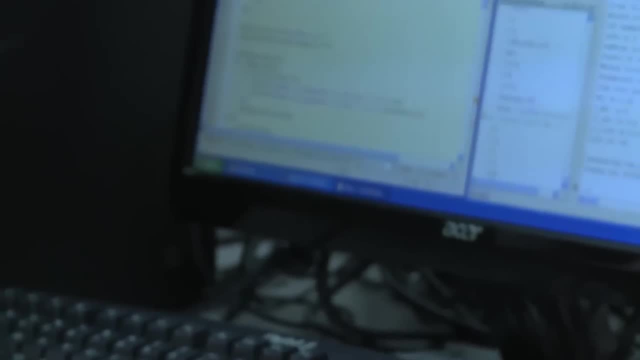 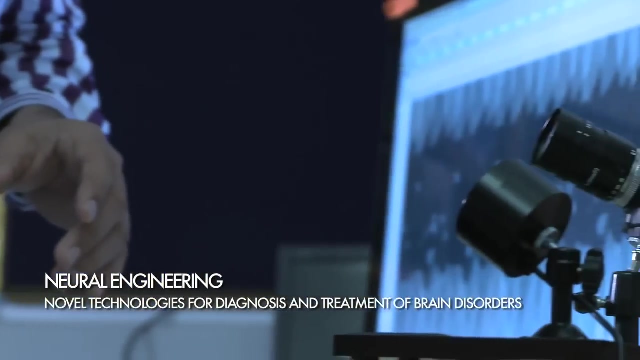 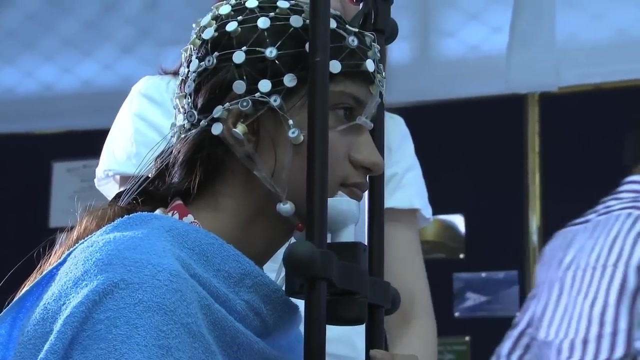 This program is designed to analyse data obtained from imaging scans of human and mice. It helps to critically evaluate the drug efficacy for cancer anti-angiogenic therapy. In the area of neural engineering, we collaborate with the Massachusetts General Hospital and Harvard Medical School in Boston. 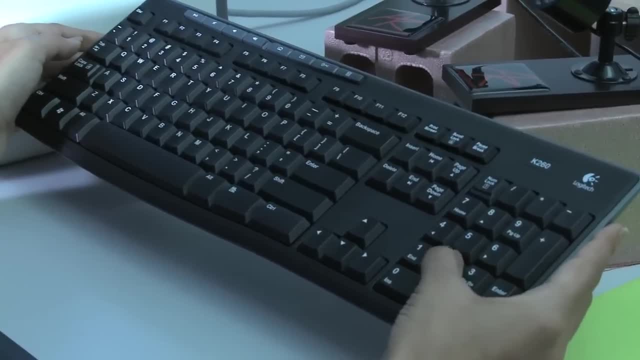 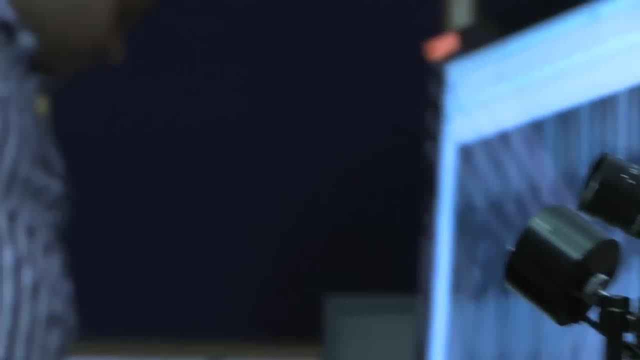 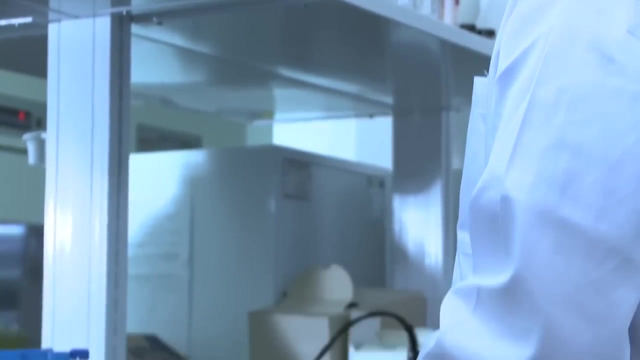 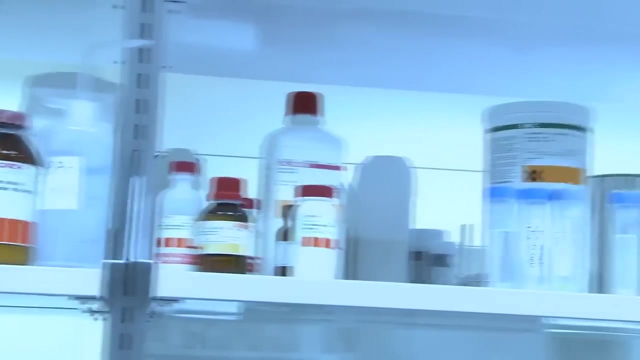 to develop novel technologies for diagnosing and treating brain disorders such as epilepsy, stroke and Alzheimer's disease. With our dedicated research team, Valence strives to become a reputable international hub on biomedical and biorelated research, where innovative idea develops into a comprehensive solution. 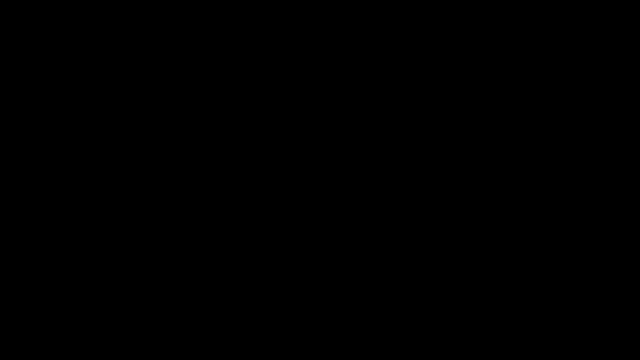 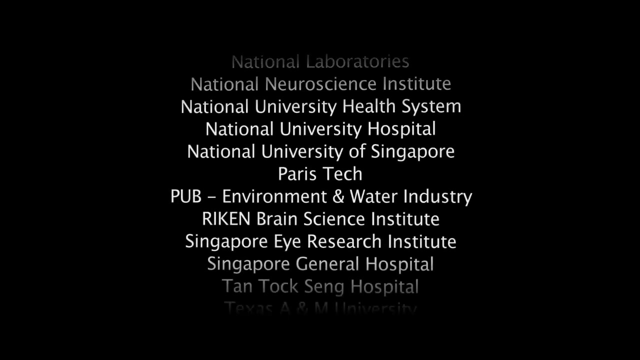 wwwvalencecom. wwwvalencecom.